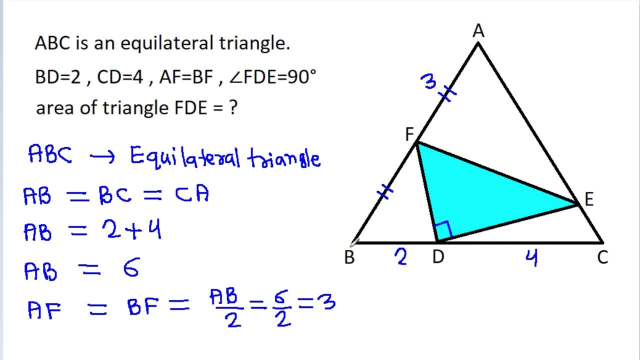 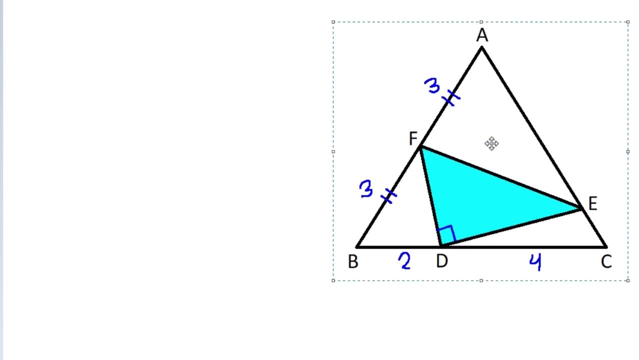 So AF will be equal to 2. be 3 and BF will be 3, and also these angles, they will be 60 degree. and suppose this angle is theta, this angle is beta and this angle is alpha, this angle is gamma. then theta plus 60 degree, plus alpha, it will be equal to 180. 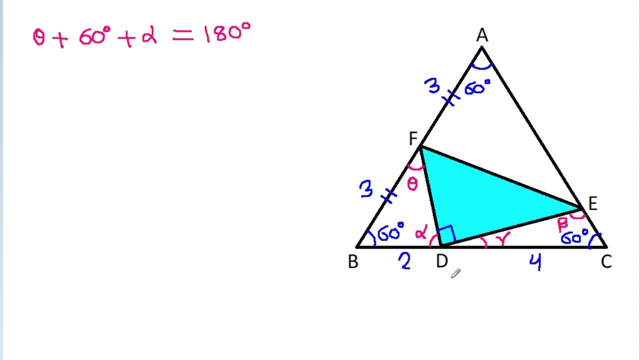 degree, and also in triangle DEC: beta plus 60 degree plus gamma, it will be equal to 180 degree. and if we add both equations, then theta plus beta plus 60 degree plus 60 degree will be 120 degree. plus alpha plus gamma, it will be equal to 360 degree. and theta: 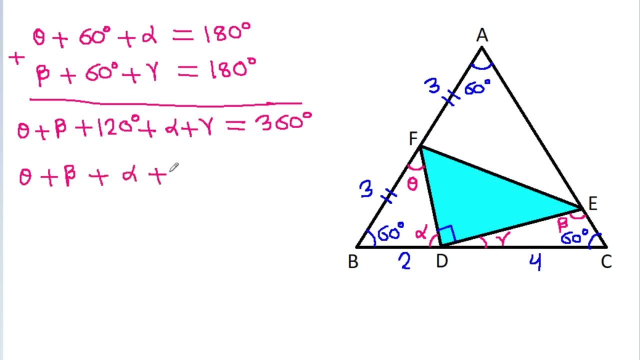 beta plus beta plus alpha plus gamma, it will be equal to 240 degree. and also alpha plus 90 degree plus gamma, it will be equal to 180 degree, because 8 point D, this angle is alpha, this angle is 90 degree and this angle is gamma, So alpha. 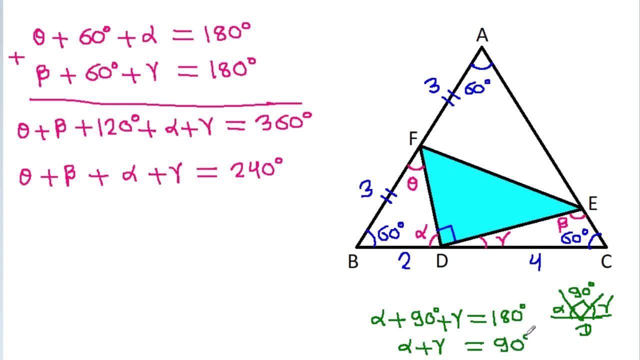 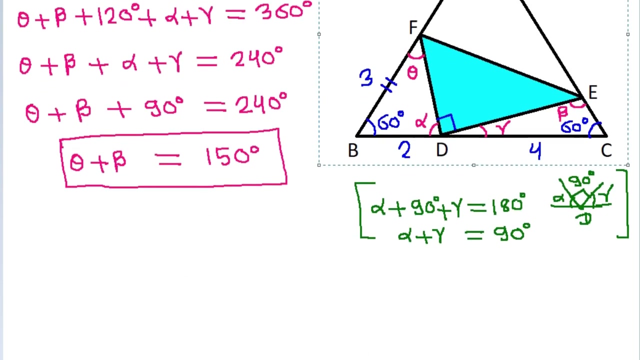 plus gamma, it will be equal to 90 degree. So theta plus beta plus 90 degree it is equal to 240 degree. So theta plus beta, it will be equal to 150 degree. And, and, and, and, and, and. 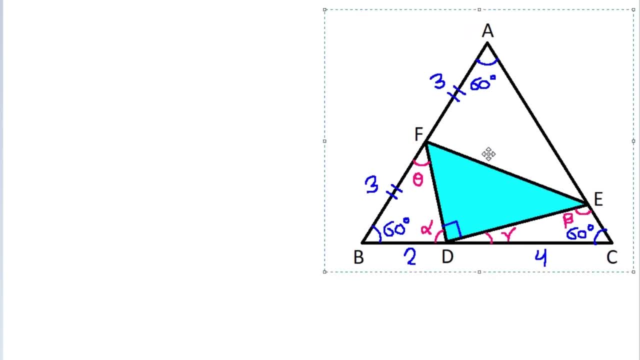 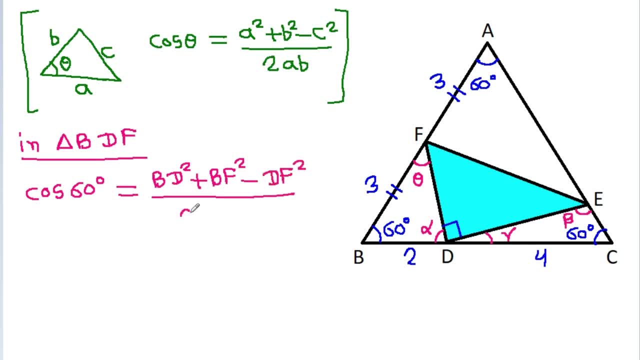 DF square by 2 times BD times BF, And suppose DF is A and DE is B, Then cos 60 degree it is 1 by 2.. That is equal to BD is 2.. S square plus BF is 3.. S square minus DF is A. S square by 2 times BD is 2 times BF is. 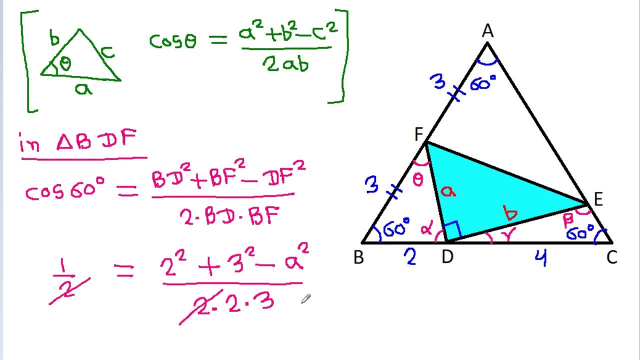 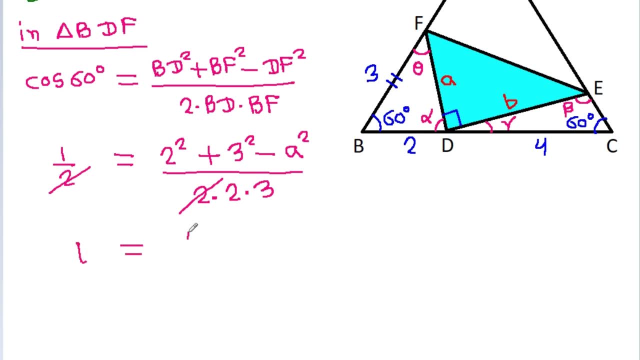 3. And 1, 2 will get cancelled. So 1 is equal to 4 plus 9 minus BF is 3.. So 1 is equal to 4 plus 9 minus BF is 3.. So 1 is equal to 4 plus 9 minus BF is 3.. 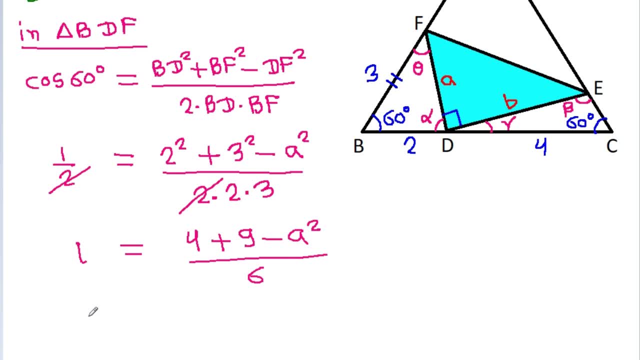 So 1 is equal to 4 plus 9 minus A square by 6.. And 6 will be equal to 13 minus A square. That means A square. it will be equal to 7.. So A will be equal to a square root of 7.. 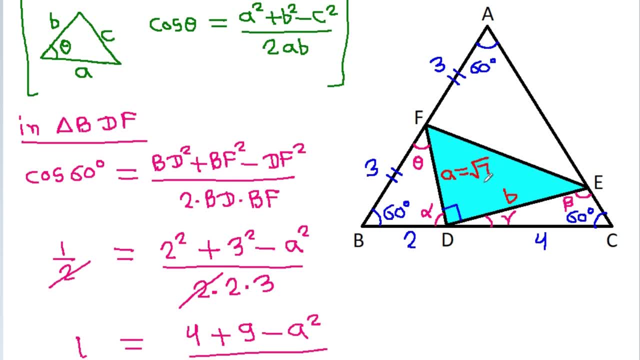 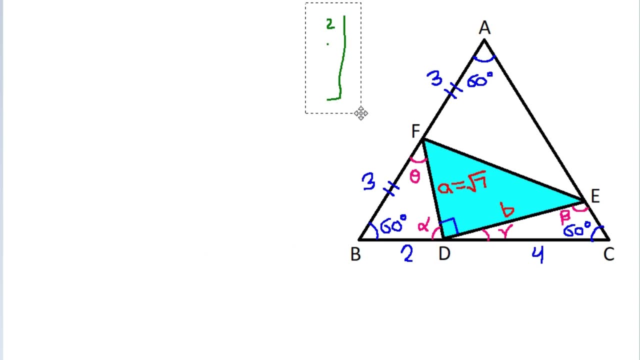 A is equal to a square root of 7.. Now in any triangle, A, B, C, if B, C is A, A, C is B and A, B is C, then A by sin A, it is equal to B by sin B, it is equal to C by sin C. 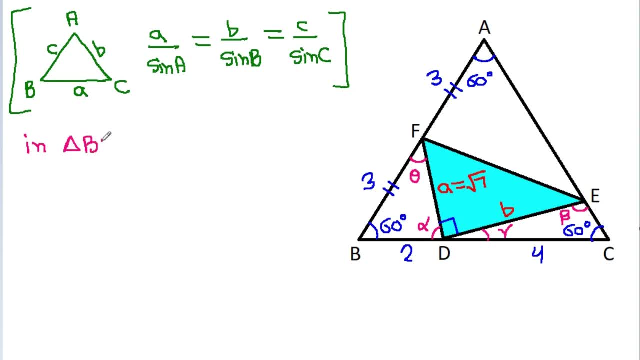 So in triangle B, D, F, D, F, D, F, by sin 60 degree it will be equal to B, D by sin theta, And D, F is a square root of 7 by sin 60 degree is a square root of 3 by 2.. 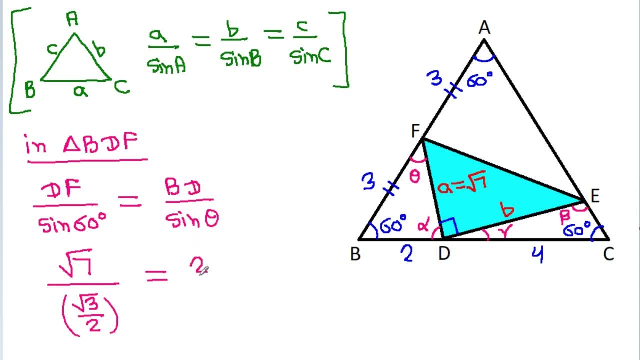 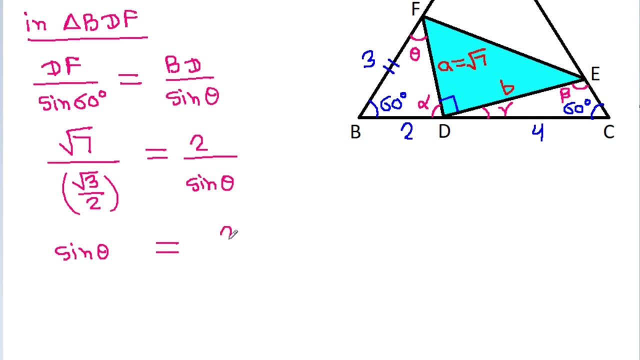 It is equal to B D. So sin theta is 2 by sin theta And sin theta it will be equal to 2 times a square root of 3 by 2 by a square root of 7.. And 2 will get cancelled. 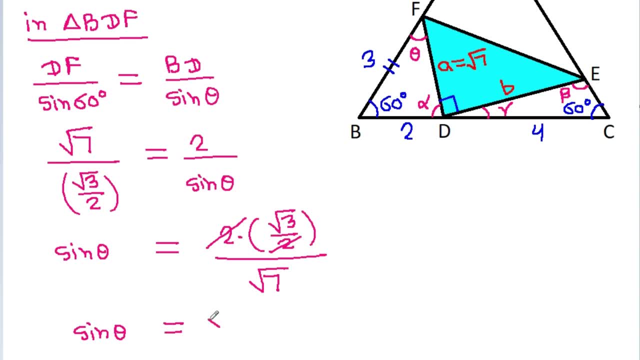 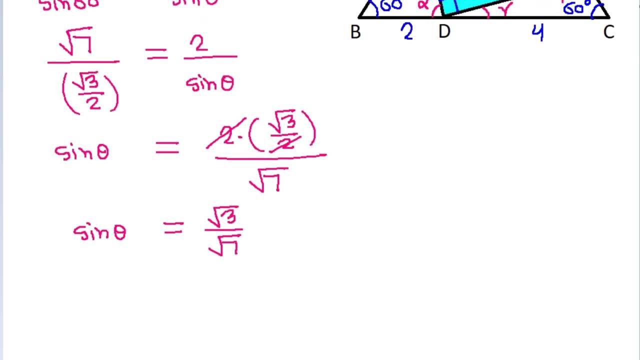 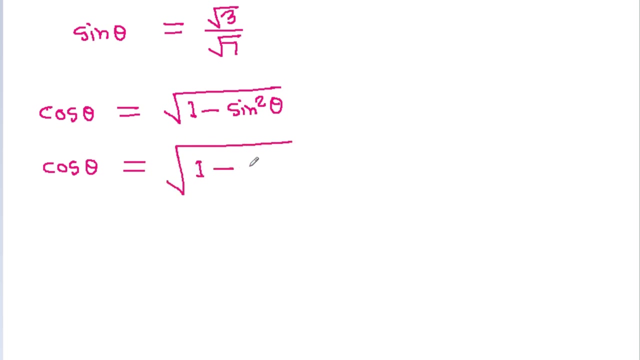 So sin theta, it is equal to a square root of 3 by a square root of 7.. And cos theta, it is equal to a square root of 1 minus. sin square theta, So cos theta, it will be equal to a square root of 1 minus. 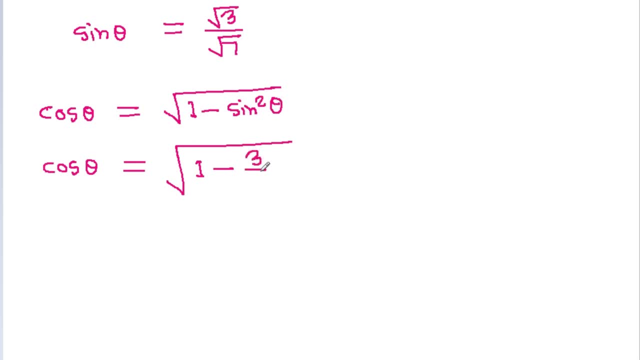 and sin square, it is equal to sin square. theta, It will be 3 by 7.. So, cos theta, it is equal to a square root, and 1 minus 3 by 7 will be 4 by 7.. 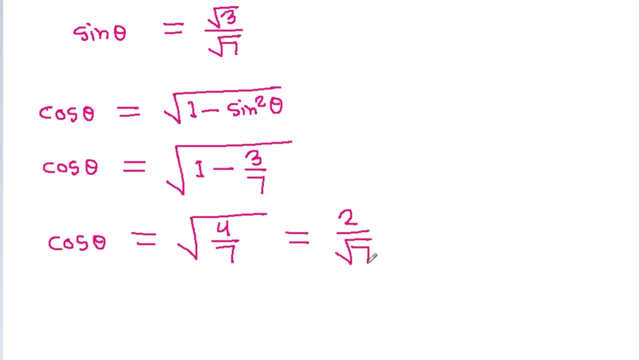 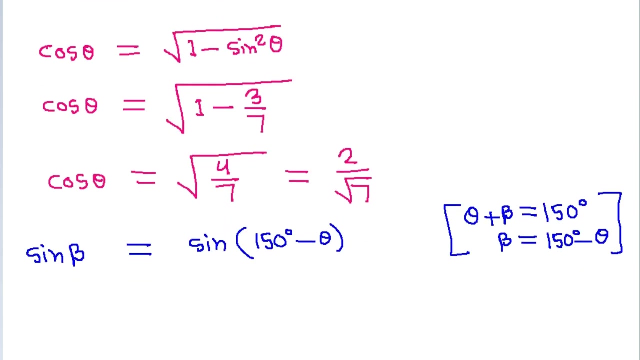 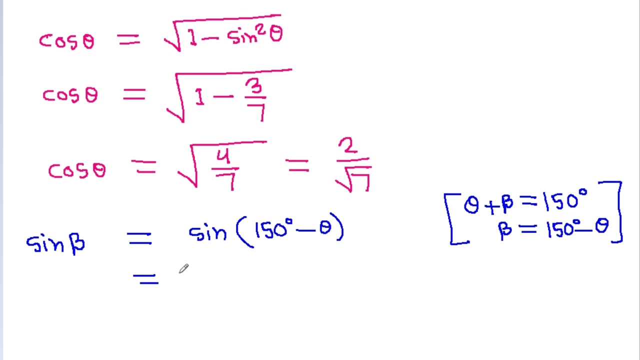 And it is 2 by a square root of 7.. So sin beta it will be equal to sin 150 degree minus theta, because theta plus beta it is 150 degree. so beta will be equal to 150 degree minus theta and sin 150 degree minus theta it will be. 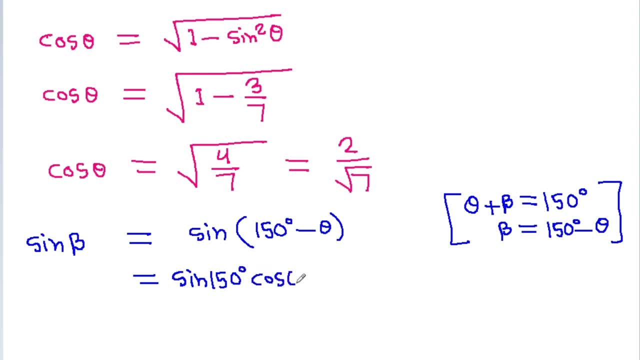 sin 150 degree, cos theta minus cos 150 degree, sin theta and sin 150 degree it is 1 by 2 times cos theta is 2 by s square root of 7 minus, and cos 150 degree is minus s square root of 3 by 2 times and sin theta it is a square root. 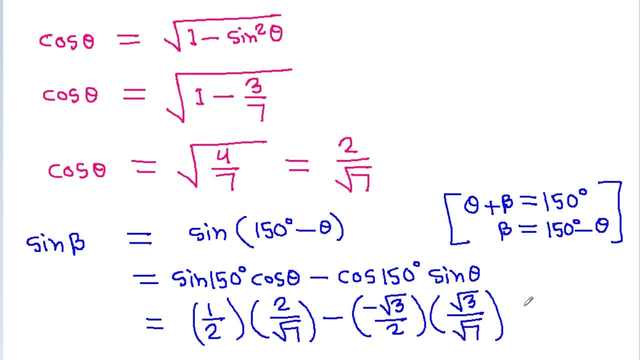 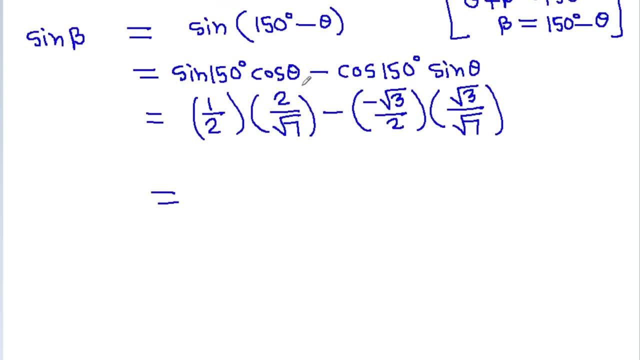 of 3 by s square root of 7, and it is equal to 2, will get cancelled. so it is 1 by s square root of 7 and minus times minus will be plus and s square root of 3 times s square root of 3 will be 3 by 2. 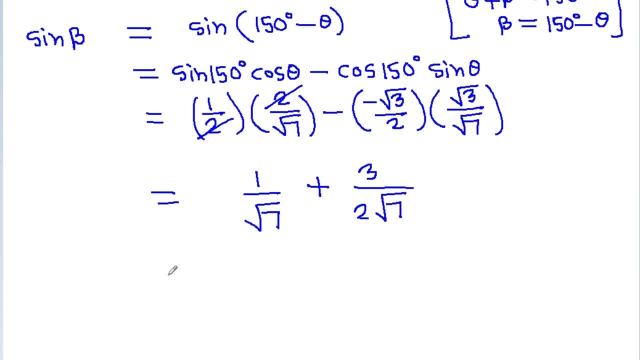 times s square root of 7, and it is 1 by s square root of 7 times 1 plus 3 by 2, that is equal to 5 by 2 times 1 by s square root of 7, and it is 5 by 2 times s square root of 7. it is sin, beta and. 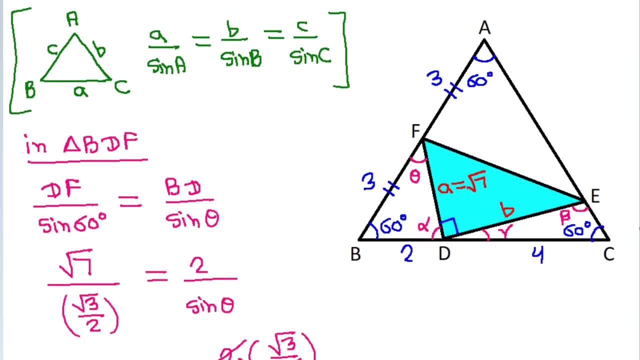 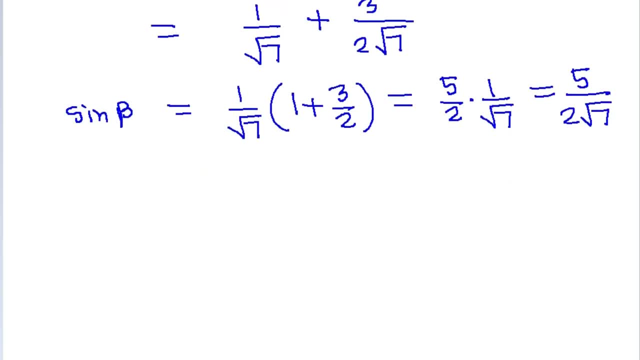 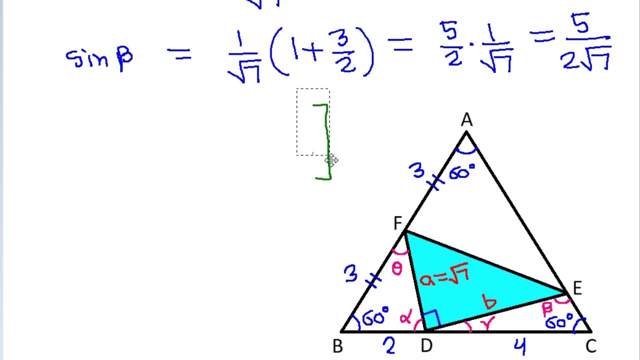 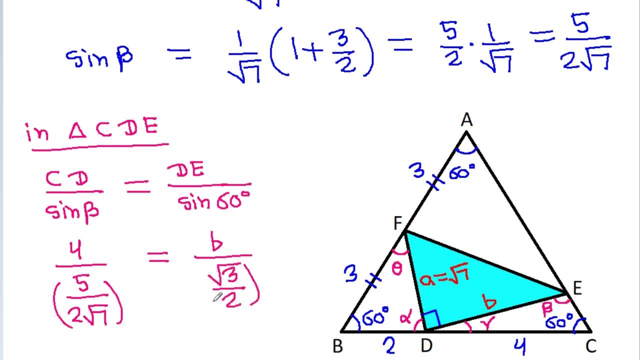 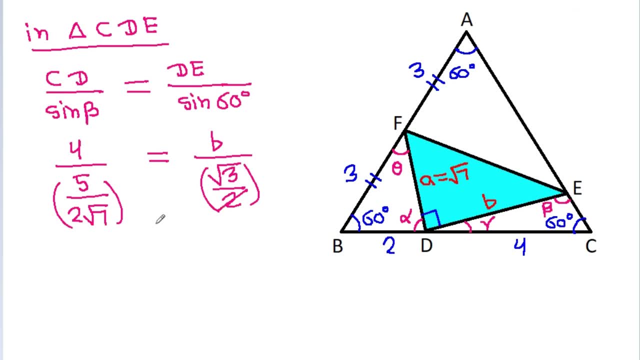 degree is a square root of 3 by 2 and 2 will get cancelled and it is 4 times a. square root of 7 by 5 is equal to B by a square root of 3, so B will be equal to 4 times a square root of 7. 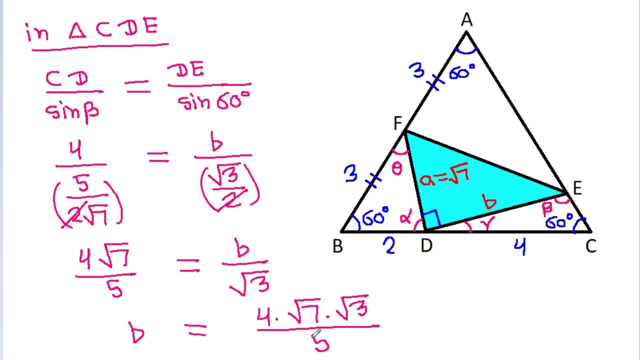 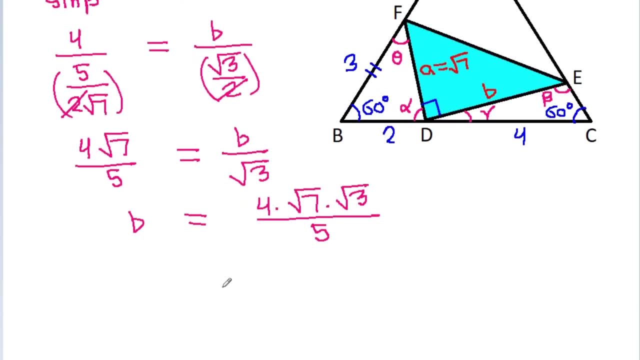 by 2.. times a square root of 3 by 5, and now area of FDE, it will be equal to 1 by 2 times base is B times height is A, and it is 1 by 2 times B is 5.. 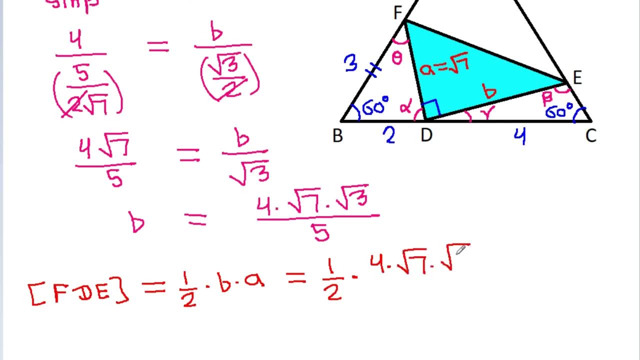 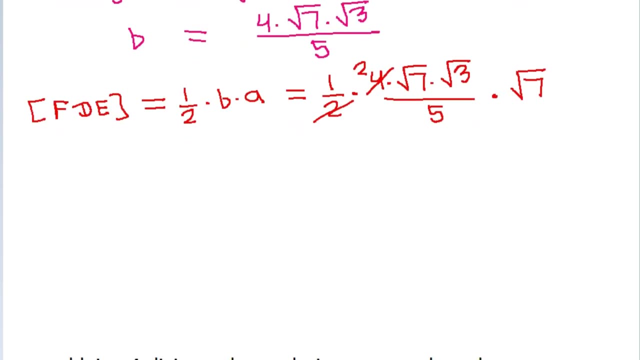 4 times a square root of 7 times a square root of 3. by 5 times A is a square root of 7 and 2 times 2 is 4, so it is equal to 2 times and a square root of 7 times a square root of 7 will be 7..